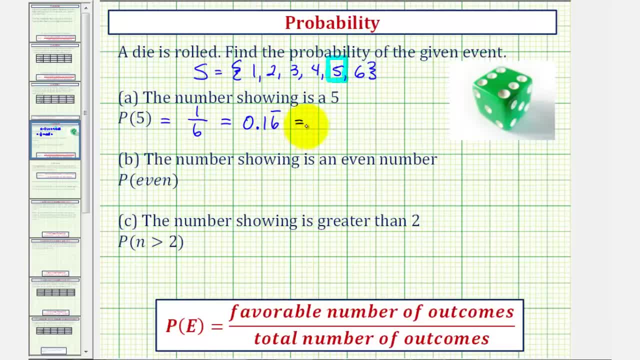 add a percent sign which would give us notice. again, the six is repeating, so we'd have sixteen point six repeating percent. We can also move the decimal point to the right two places and add a percent sign. Next I want to determine the probability. the number showing is an even number. 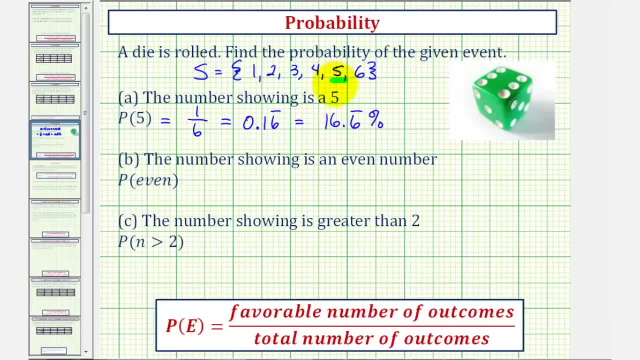 Even numbers are divisible by two. so, again looking at our sample space, we have three favorable outcomes: the two, four or six, And therefore the probability of rolling an even number would be equal to three sixths or three divided by six, which does simplify to one-half. 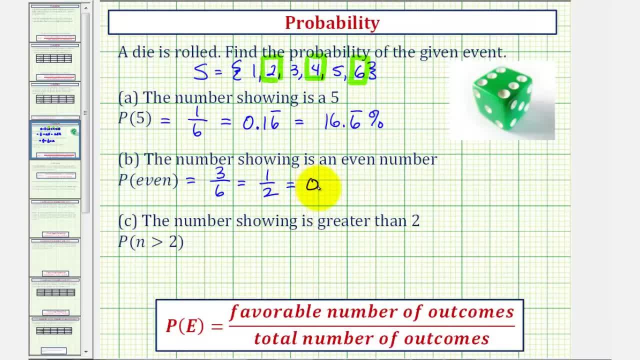 which we should recognize as a decimal, as zero point five, and as a percentage- 50%. And then, finally, we want to determine the probability. the number is showing is greater than two. We need to be a little careful here, Notice: two is not greater than two. 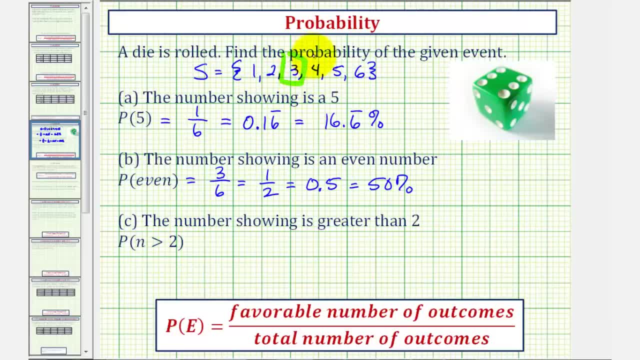 so the favorable outcomes would be three, four, five and six. So there are four favorable outcomes out of six total outcomes and therefore the probability of the number being greater than two is equal to four. six, which simplifies to two thirds. 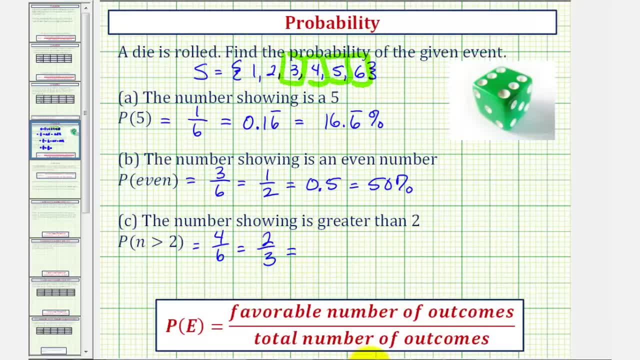 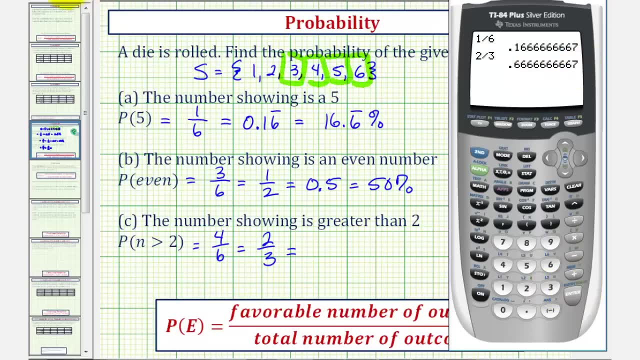 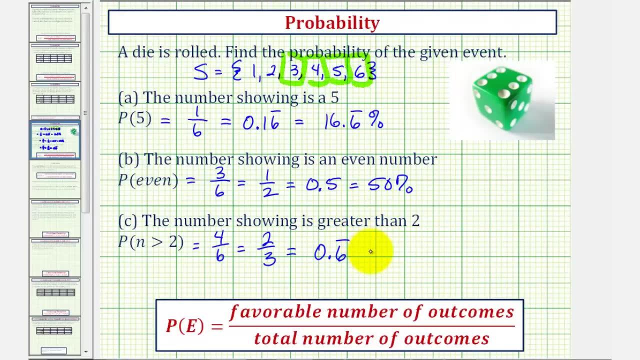 We should recognize this as point six repeating. but let's go ahead and verify that Two divided by three is point six repeating. So as a decimal we would have zero point six, with a bar over the six showing the six repeats, and as a percentage we would have: 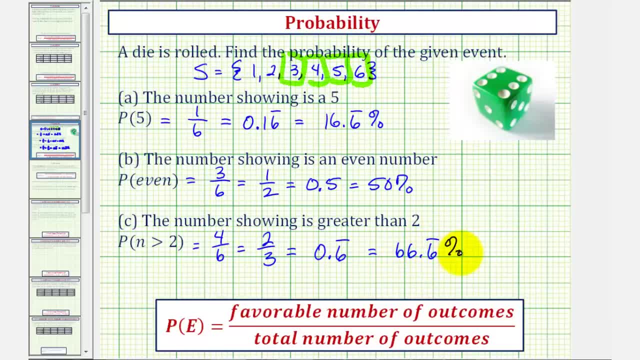 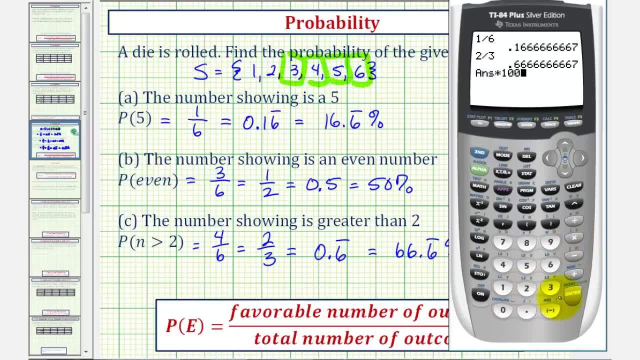 66.6. repeating percent. Notice how. if we go back to the calculator just for a moment, if we multiply this by 100, it does convert the decimal to a percent. We just have to remember to add the percent sign. We also need to recognize the six is repeating. 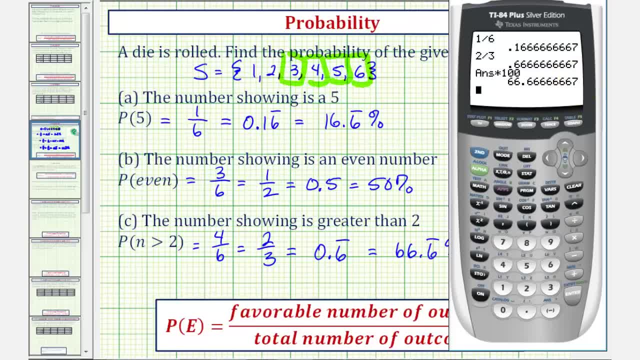 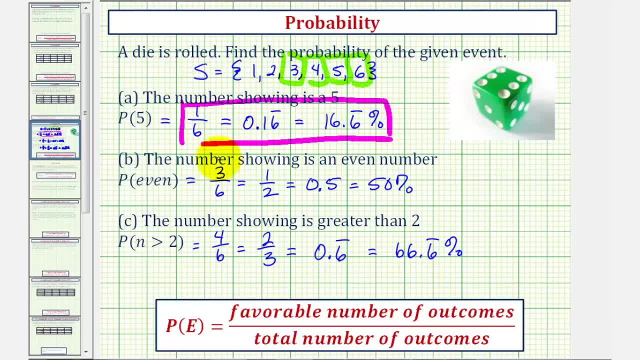 even though the calculator is rounding here on the far right. So here we expressed each probability as a fraction, decimal and percentage. Just be sure, if your question indicates the probability in a specific way, you do so. I hope this was helpful.